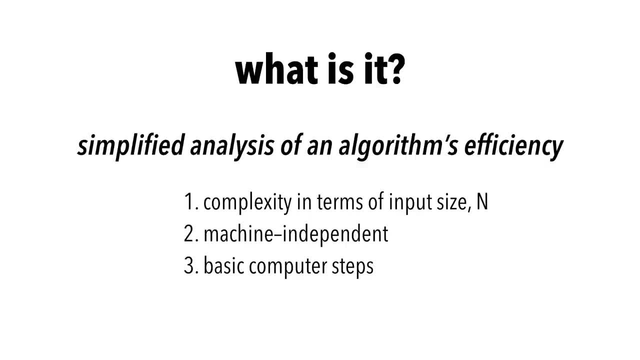 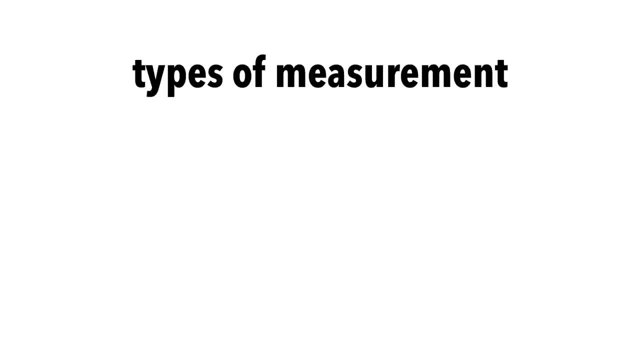 computer steps of the code. We can use Big O to analyze both time and space. There are a couple ways to look at an algorithm's efficiency. We can examine worst case, best case and average case. When we're talking Big O Notation, we typically look at worst case. 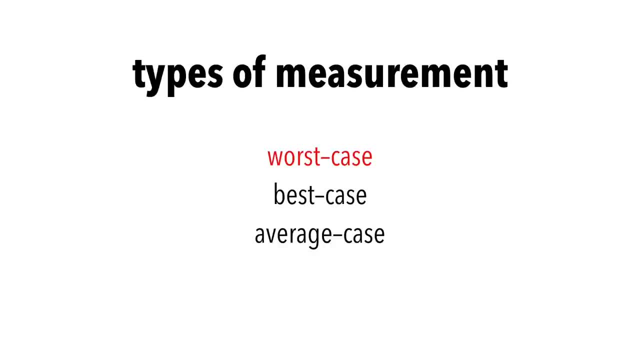 This isn't to say the others are unimportant. however, Let's talk about a few rules First. Big O Notation ignores constants. For example, if you have a function that has a running time of 5n, we say that it runs on the order of Big O. 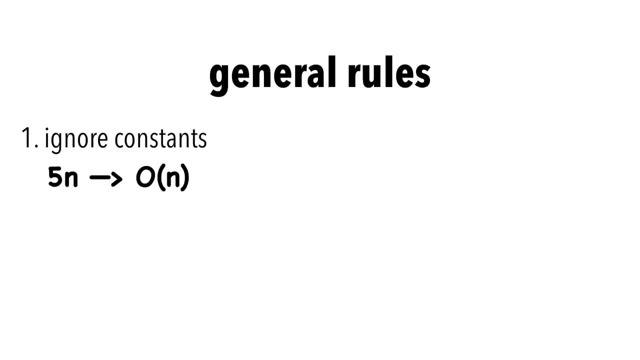 This is because, as n gets large, the 5 no longer matters. In the same way as n grows, certain terms dominate others. Here's a list, but I'll show you how to do it. I'll give you a visual on the next page. 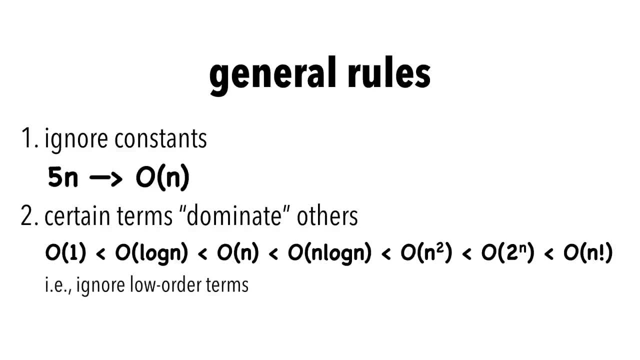 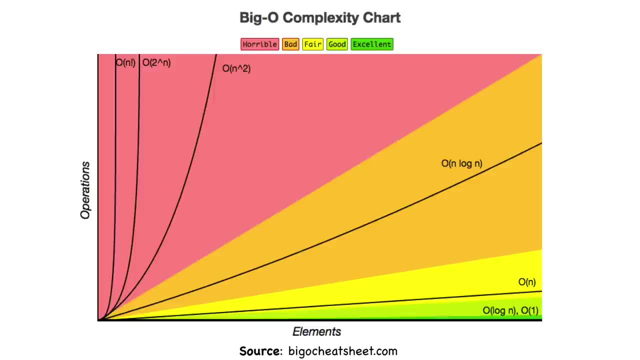 We ignore or drop low-order terms when they're dominated by high-order ones. Take a minute and study this chart. It can be found on BigOCheatCheatcom, along with a handy guide on the Big O of various important algorithms. Let's run a few examples so you can see what I mean by basic computer steps. 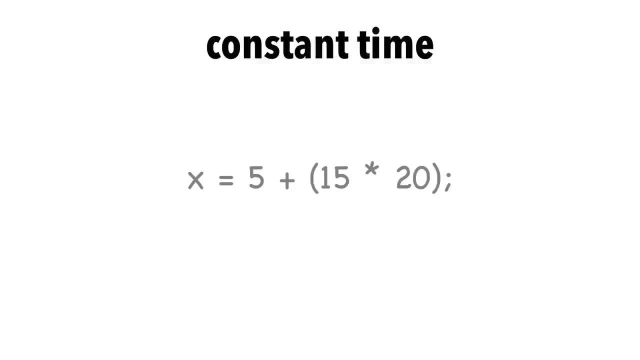 We'll start with constant time. Imagine we have the following line of code: This basic computer statement computes x and notice it does not depend on the input size in any way. We say this is Big O or constant time. What happens when we have a sequence of statements? 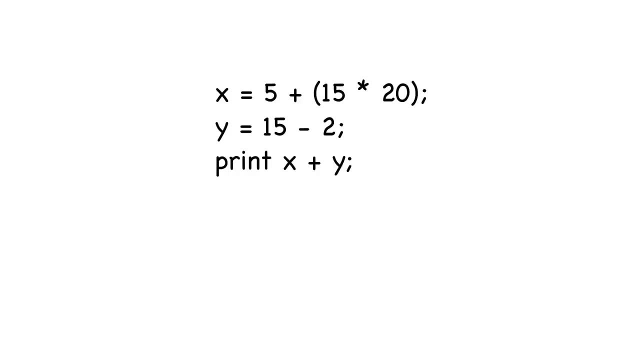 Notice that all these are constant time. How do we compute Big O for this block of code? We simply add each of their times and we get 3 multiplied by Big O of 1.. But remember we dropped constants, so it's still Big O of 1.. 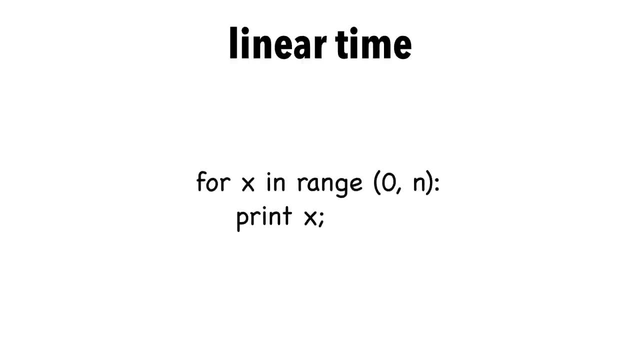 Let's look at linear time. Suppose we have the following for loop that prints the numbers 0 to n. We know the print statement is Big O of 1.. This means the block of code is n times Big O of 1, in other words, Big O of n. 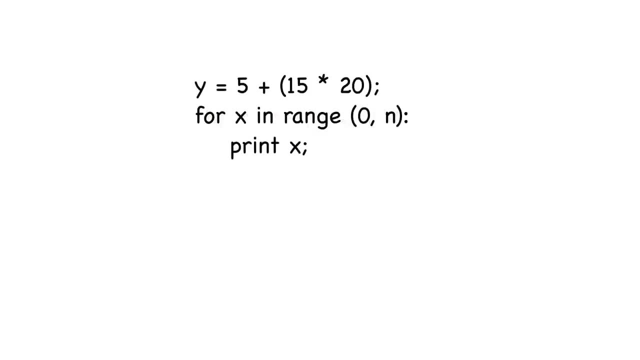 Here's another sequence. The first line we know again is Big O of 1, and the for loop is Big O of n. The total time is the summation of these two, but remember we dropped low order terms. When n gets large, the time it takes to compute y is meaningless. 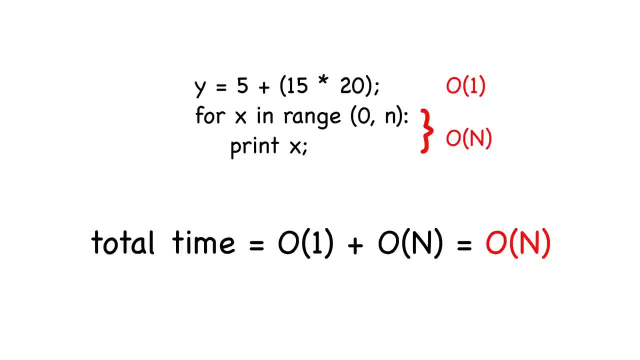 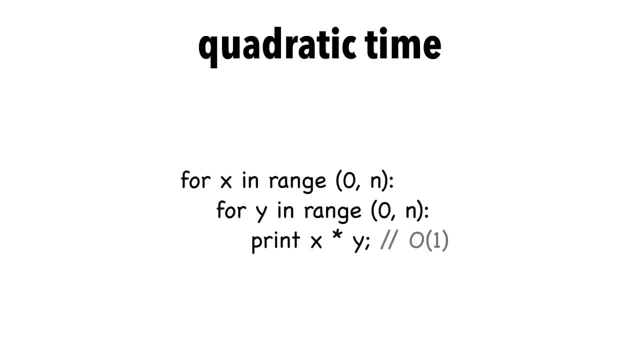 as the for loop dominates the run time. Finally, let's look at quadratic time. The first line we know again is Big O of 1, and the for loop is Big O of n. I think you can see that the print statement will be executed n times n. 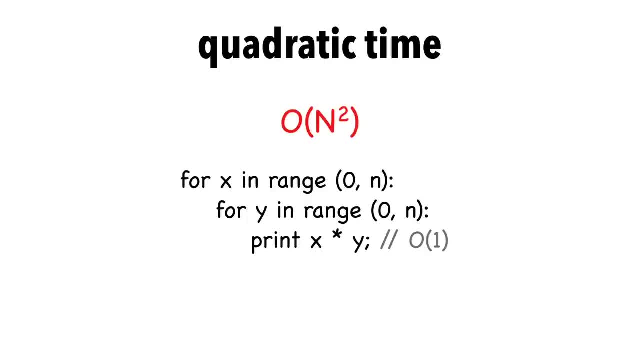 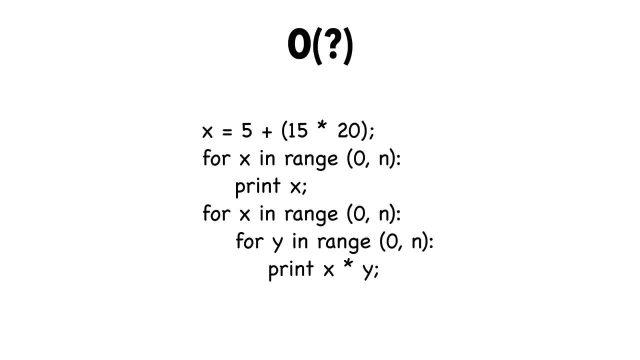 which gives us Big O of n squared. Let's do two more examples covering everything we've talked about. Say, we have the following block of code: What is its total run time? Well, we know the run time for each of these. 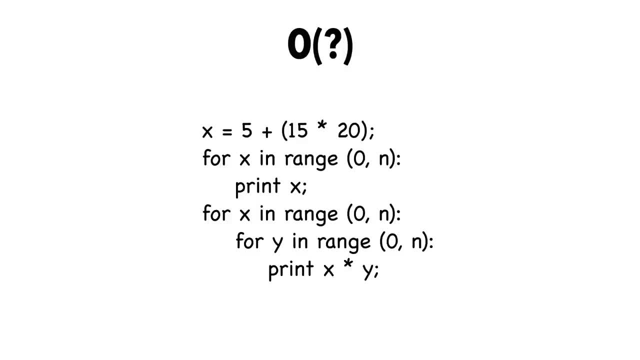 so the total run time is simply the max of the three. Now let's look at the big O of n squared. The nested for loop dominates here, so we get Big O of n squared. How about this if-else statement Pretend? the sequence of statements in each clause have already been deduced to the Big O, as shown. 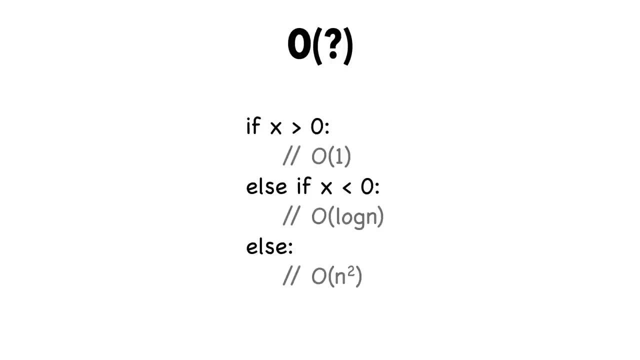 We talked earlier that when we're discussing Big O, we usually look at worst case scenario. So for this situation we choose the largest run time, which happens to be Big O of n squared. I hope this gives you an understanding of Big O notation. 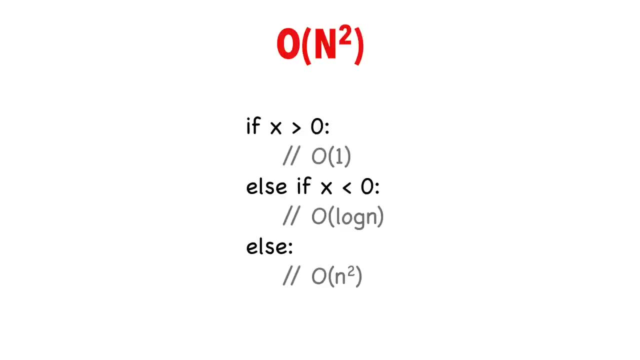 Let's wrap up by talking about the real world. When you're coding your algorithm, please realize that constants absolutely do matter. A lot of situations have small input sizes, so a constant of 2 or 3 could have a large impact. Lastly, for the same reason, be cognizant of best and average case. 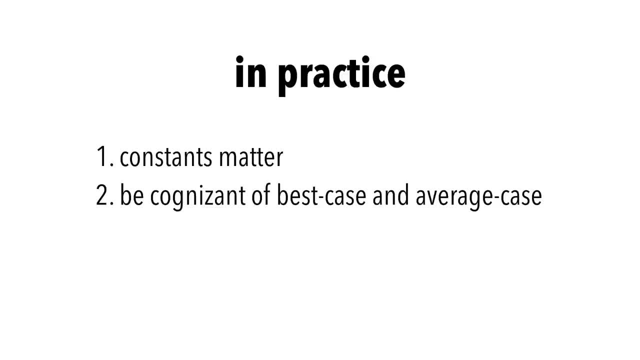 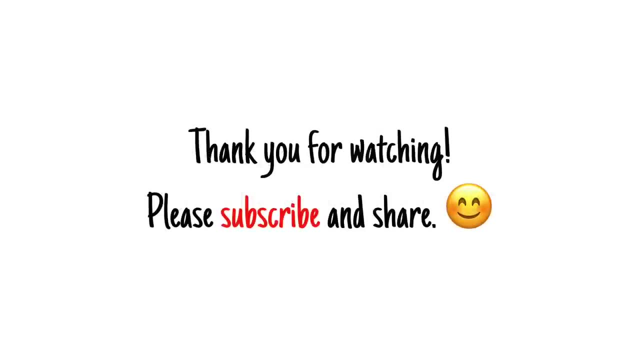 Depending on your application, this may be more applicable for your algorithm. As always, thank you for watching. Please subscribe if this helped you.